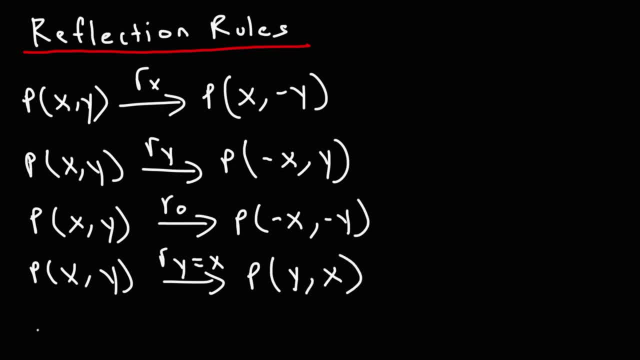 So x, y, Y becomes y, x. Now, if we wish to reflect a point across the line, y equals negative x. we're going to switch x and y, like we did before, but we're also going to negate each variable. 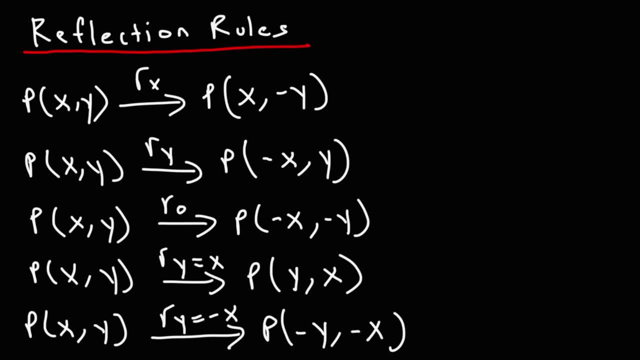 So, rather than being positive y, positive x, it's going to become negative y, negative x. So those are some reflection rules that you want to be familiar with. Feel free to write this down in your notes somewhere, because we're going to use this shortly. 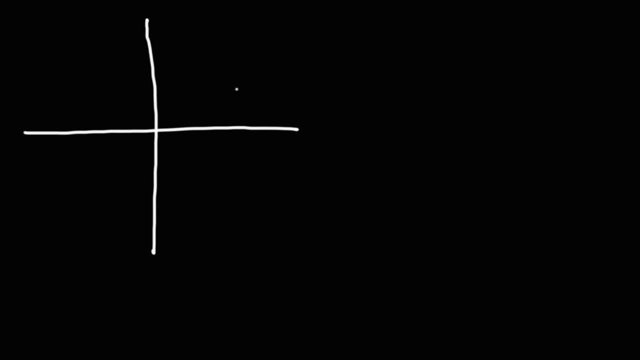 So let's say we have the point 3,2.. Let's say it's somewhere in this region. What's going to be the reflected point if we reflect it over the x-axis? So here is the x-axis. Notice that we have a point 3,2.. 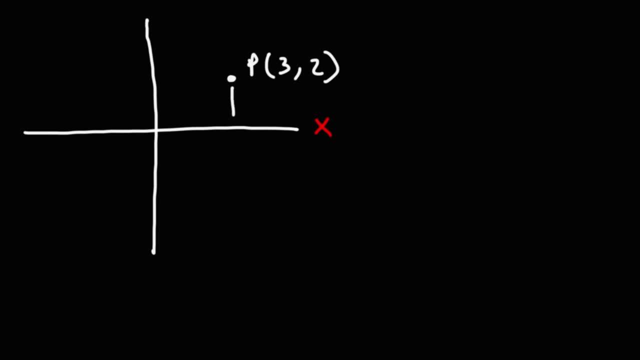 Notice that we have to travel two units to get from the point to the x-axis. To get the reflected point, we need to draw the reflection. So it's going to be over here. The new point is going to be: it's going to have the same x value. 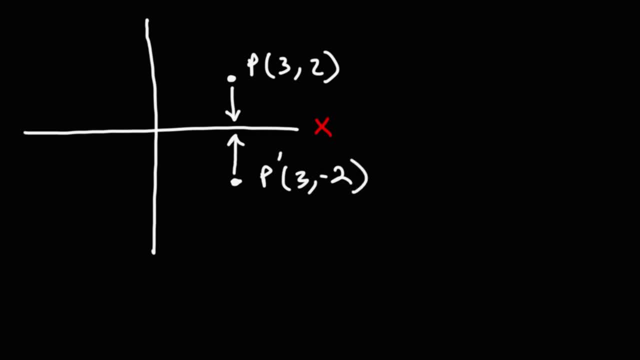 but the y value is going to change from positive 2 to negative 2.. So that's the reflected point across the x-axis. Now what if we want to reflect the original point About the y-axis instead? Notice that we have to travel three units to go from that point to the y-axis. 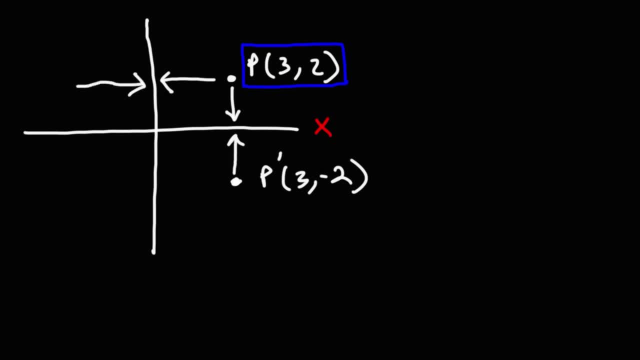 Therefore, the reflected point is also going to be three units from the y-axis as well, So it should be somewhere in this region. Now, this time the y value is going to stay the same, but the x value is going to change from positive 3 to negative 3.. 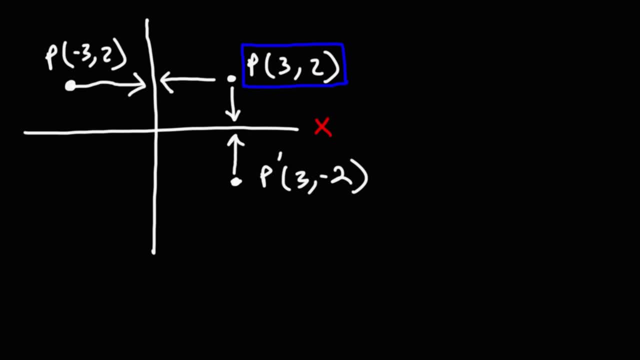 So it's going to be negative 3,2.. Now what if we want to reflect that point across the origin, So we have to travel this distance to get from the first point to the origin? The reflected point is going to be the same. 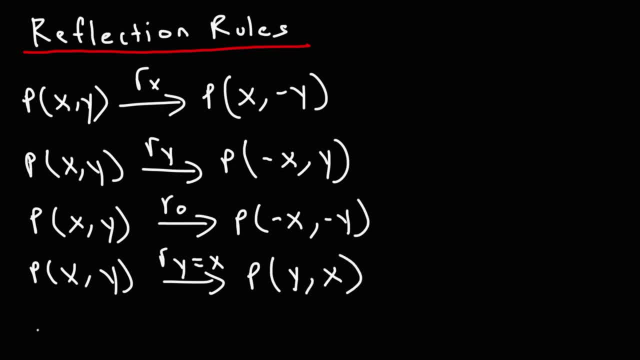 So x, y, Y becomes y, x. Now, if we wish to reflect a point across the line, y equals negative x. we're going to switch x and y, like we did before, but we're also going to negate each variable. 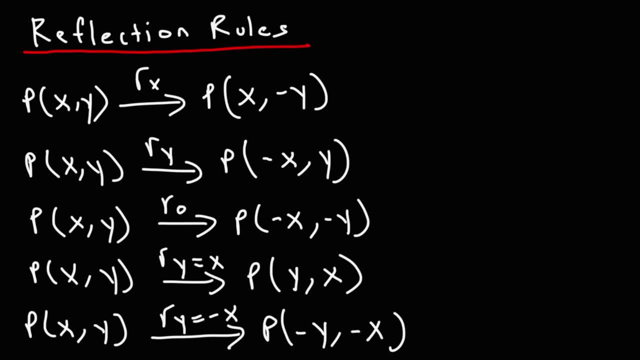 So, rather than being positive y, positive x, it's going to become negative y, negative x. So those are some reflection rules that you want to be familiar with. Feel free to write this down in your notes somewhere, because we're going to use this shortly. 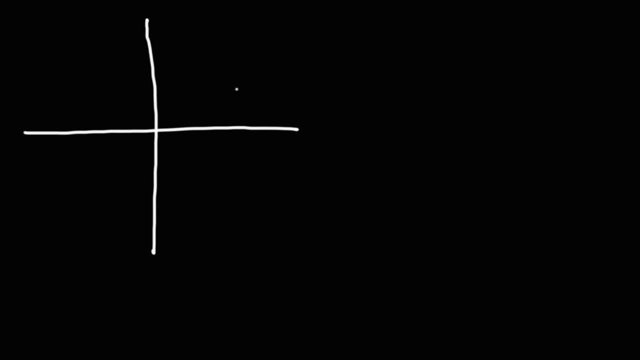 So let's say we have the point 3,2.. Let's say it's somewhere in this region. What's going to be the reflected point if we reflect it over the x-axis? So here is the x-axis. Notice that we have a point 3,2.. 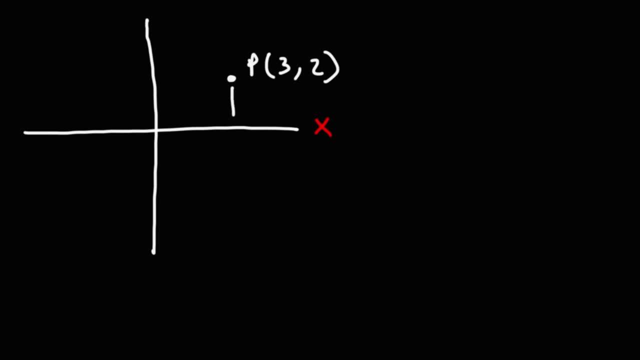 Notice that we have to travel two units to get from the point to the x-axis. To get the reflected point, we need to draw the reflection. So it's going to be over here. The new point is going to be: it's going to have the same x value. 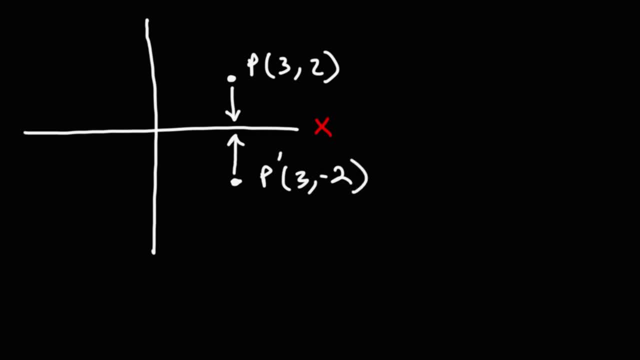 but the y value is going to change from positive 2 to negative 2.. So that's the reflected point across the x-axis. Now what if we want to reflect the original point About the y-axis instead? Notice that we have to travel three units to go from that point to the y-axis. 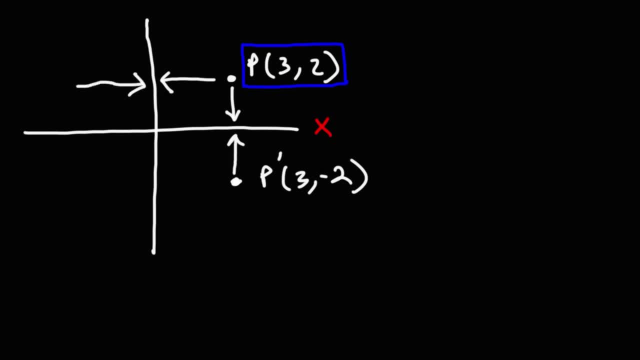 Therefore, the reflected point is also going to be three units from the y-axis as well, So it should be somewhere in this region. Now, this time the y value is going to stay the same, but the x value is going to change from positive 3 to negative 3.. 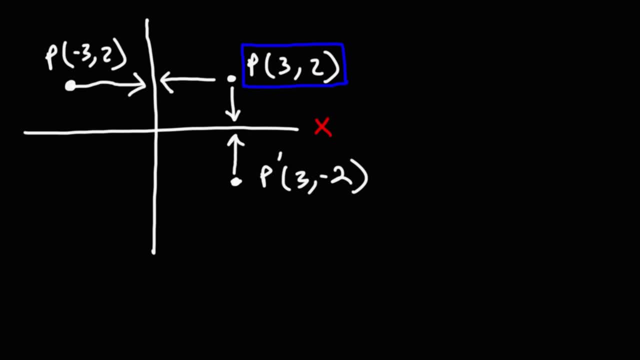 So it's going to be negative 3,2.. Now what if we want to reflect that point across the origin, So we have to travel this distance to get from the first point to the origin? The reflected point is going to be the same. 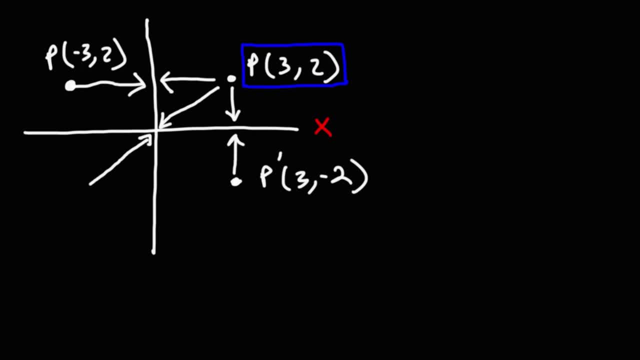 it's going to be equidistant from the origin, So it should be somewhere in this region here. Now that point. it's going to be everything that we have here, but negative. So instead of positive 3,2, it's going to be negative 3,, negative 2.. 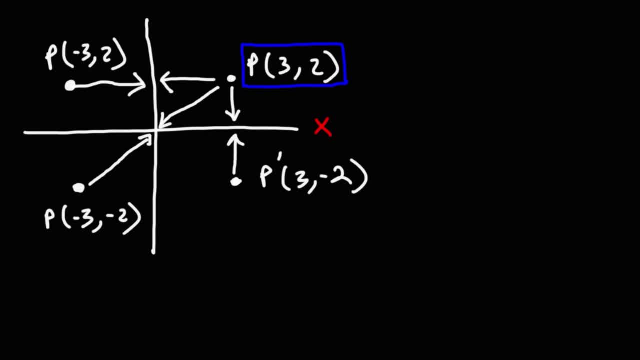 So whenever you reflect the point about the origin, both the x and the y values will change sign. Now, what about reflecting that same point but about the line y equals x? So here's the line y equals x And let's say this is 3,2.. 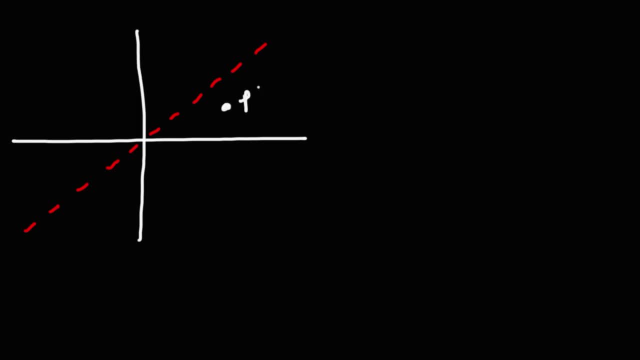 Let's say it's somewhere here. Where is the reflected point? So if we draw the shortest line that we can from the point to the line y equals x, that line will be right here. Now the reflected point is going to be across that, So it's going to be over here, but with the same distance, So it's going to be. 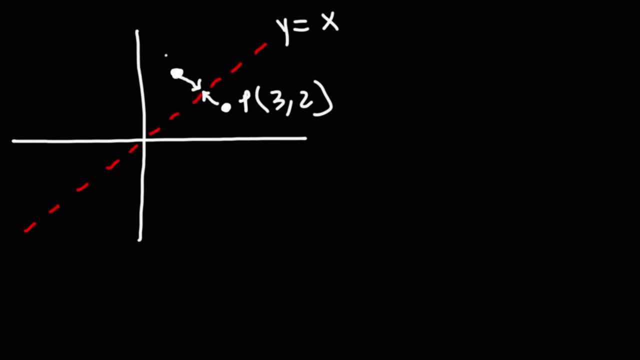 somewhere in this region. This is basically the inverse of the first point, So the x and the y values will change. This is going to have an x value of 2 and a y value of 3.. Now, my graph is not drawn to scale, but you can see how it works. It's a rough approximation, But this will be the. 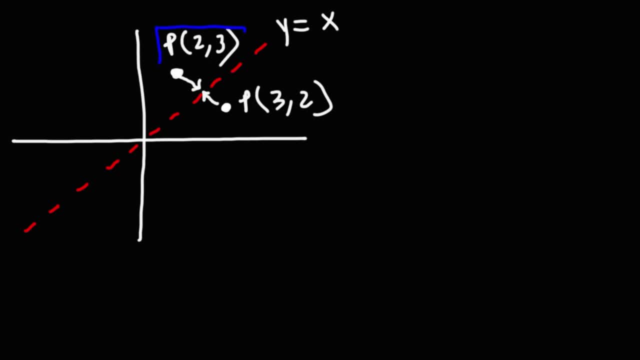 exact point. if you reflect it across the line y equals x, All you got to do is simply change x and y. Now what if we want to reflect the line y equals x? Now, what if we want to reflect the point about the line y equals negative x? 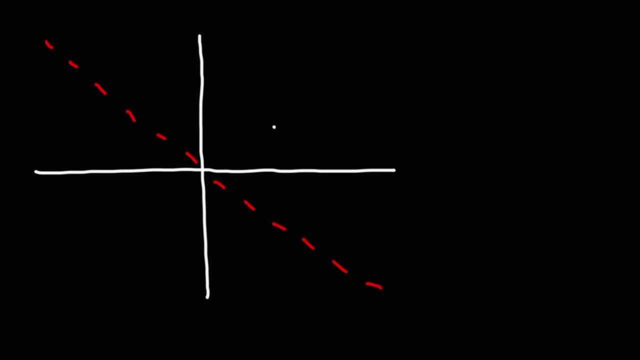 So let's say we have the same point 3 comma 2, which should be somewhere in this area, And we want to reflect it across that line. So if we want to draw a straight line from this point to the line y equals x, we would get that. 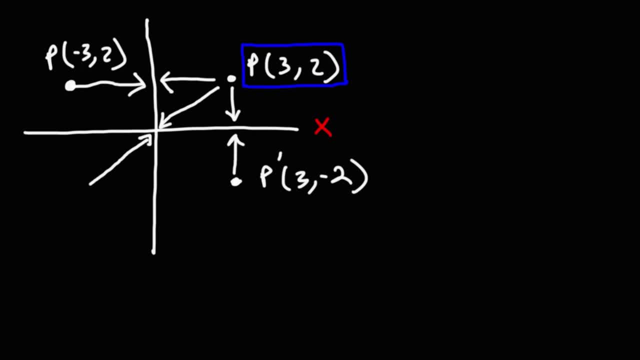 it's going to be equidistant from the origin, So it should be somewhere in this region here. Now that point. it's going to be everything that we have here, but negative. So instead of positive 3,2, it's going to be negative 3,, negative 2.. 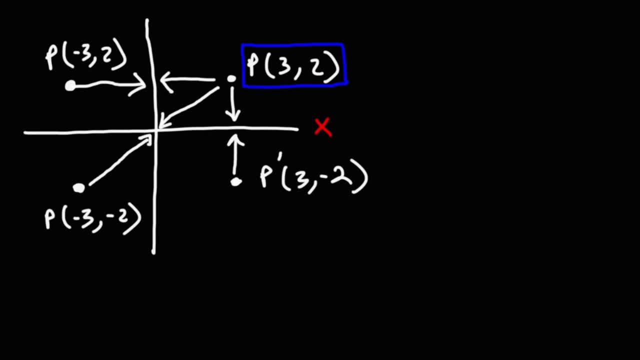 So whenever you reflect the point about the origin, both the x and the y values will change sign. Now, what about reflecting that same point but about the line y equals x? So here's the line y equals x And let's say this is 3,2.. 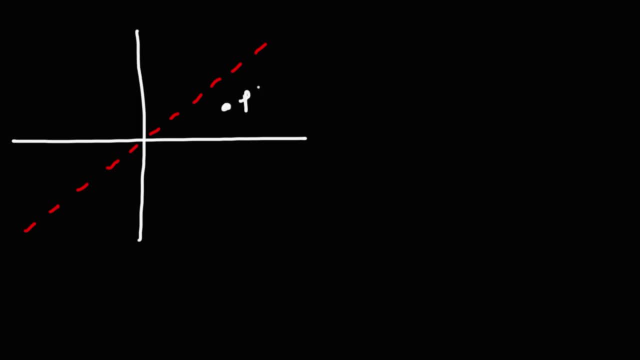 Let's say it's somewhere here. Where is the reflected point? So if we draw the shortest line that we can from the point to the line, which is the line y equals x, that line will be right here. Now the reflected point is going to be across that. 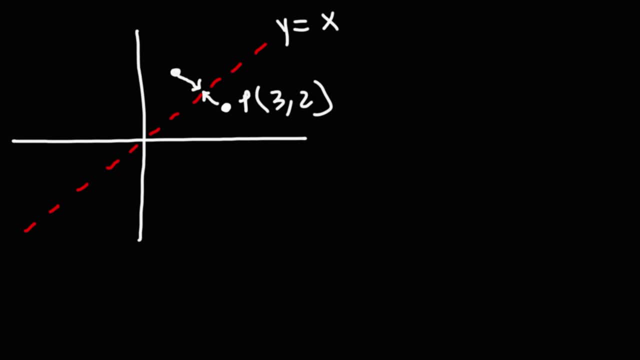 So it's going to be over here, but with the same distance, So it's going to be somewhere in this region. This is basically the inverse of the first point, So the x and the y values will change. This is going to have an x value of 2 and a y value of 3.. 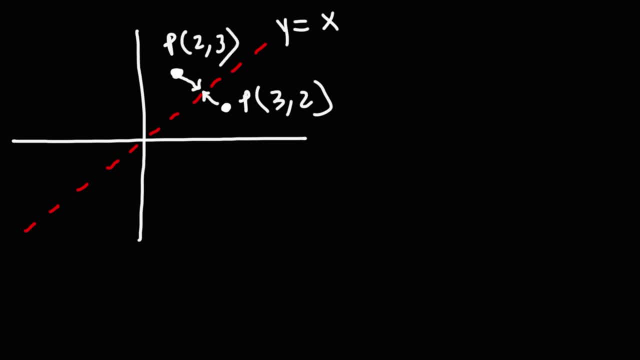 Now, my graph is not drawn to scale, but you could see how it works. It's a rough approximation, But this will be the exact point if you reflect it across the line. y equals x. All you got to do is simply change x and y. 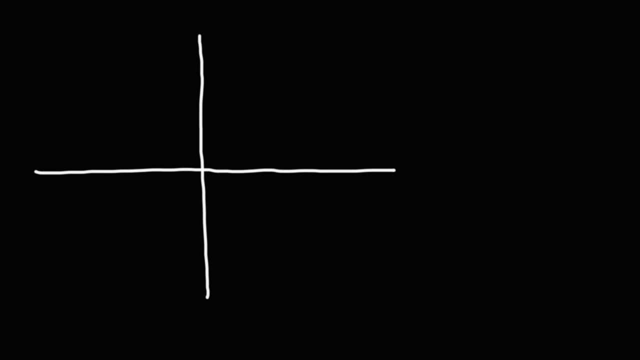 Now what if we want to reflect a point about the line y equals negative x? So let's say we have the same point- 3 comma 2, which should be somewhere in this area, And we want to reflect it across that line. 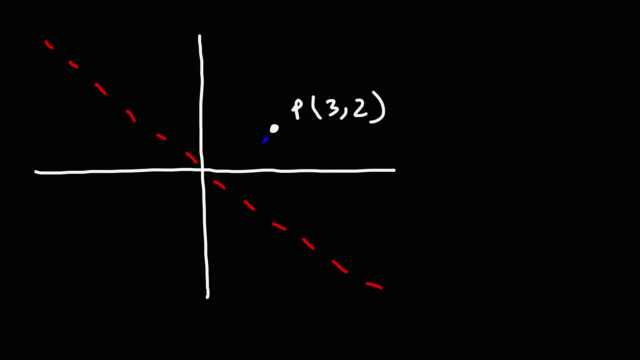 So if we were to draw a straight line from this point to the line, y equals x, we would get that. Now, if we draw the reflection of that and make sure it's the same length, we should get a point somewhere in this region. 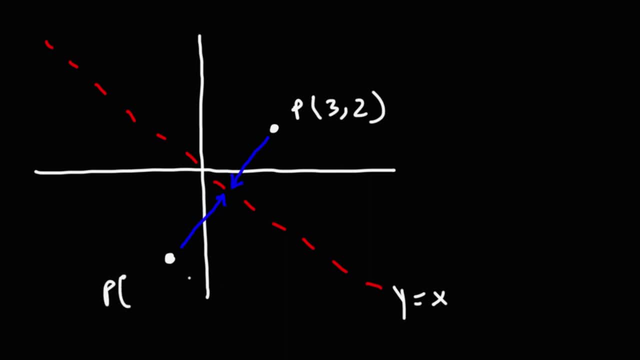 Now that point. it's going to have the same numbers- 3 comma 2, but they're going to be reversed and negated. So instead of 2, 3,, it's going to be negative 2,, negative 3.. 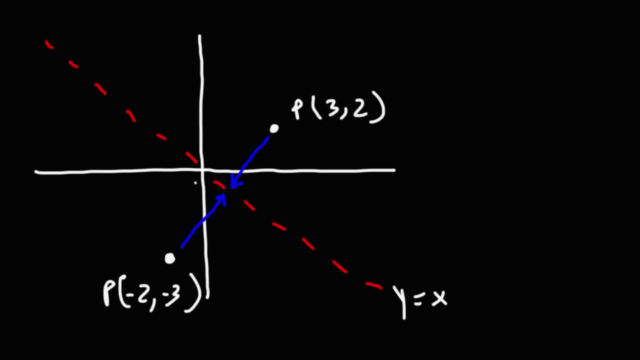 And you can kind of see that. I mean it looks like we're traveling 2 units to the left and 3 units down, But that's how you can reflect the point about the line y equals negative x. Let's put the negative sign there. 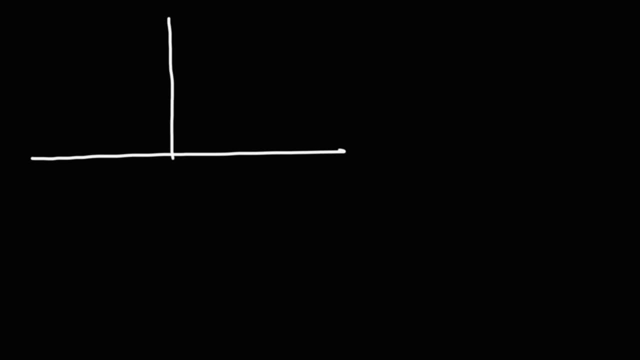 Now let's say we have the same point 3, comma 2.. Actually, let's use a different point. Let's say we have the line x equals 4, which is the vertical line, And we have the point 7, comma 3.. 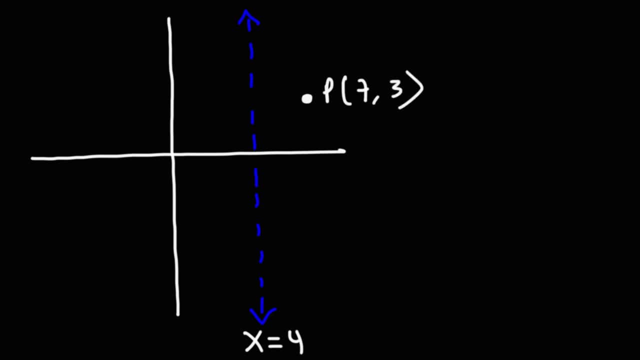 What will be the new point if we reflect that point across the line x equals 4? So that point is 3 units away from the line x equals 4.. So to draw the reflected point we need to travel 3 units across that line from it. 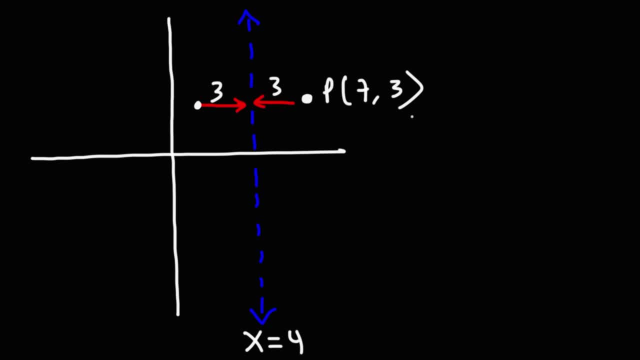 So that will take us to this point. Notice that the y values will be the same for the new point, But the x value will be different. If you want to find the new x value, there's two ways you can do this. You can take 7 and subtract it by 3, two times. 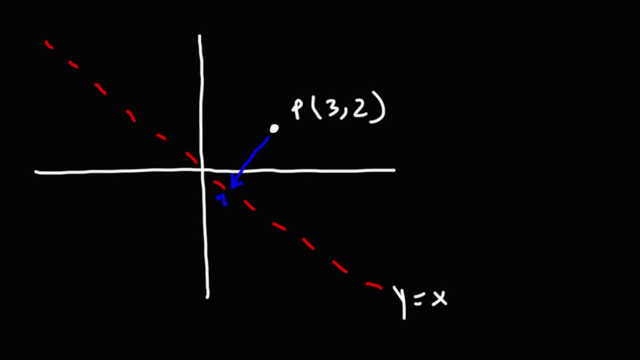 Now, if we draw the reflection of that and make sure it's the same length, we should get a point somewhere in this region. Now that point is going to be the same length as the point across the line. y equals x. that point it's going to have the same numbers- 3, 2, but they're going to be reversed and 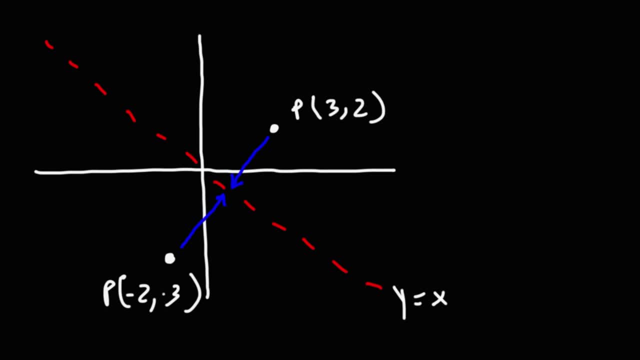 negated. So instead of 2,, 3,, it's going to be negative 2,, negative, 3.. And you can kind of see that. I mean it looks like we're traveling two units to the left and three units down, But that's how you can reflect. the point about the line y equals negative. 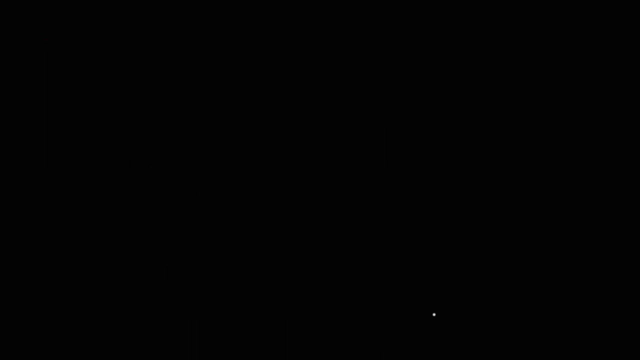 x. Let's put the negative sign there. Now, let's say we have the same point: 3, 2.. Actually, let's use a different point. Let's say we have the line x equals 4. Which is the vertical line, And we have the point 7, 3.. What will be the new point if? 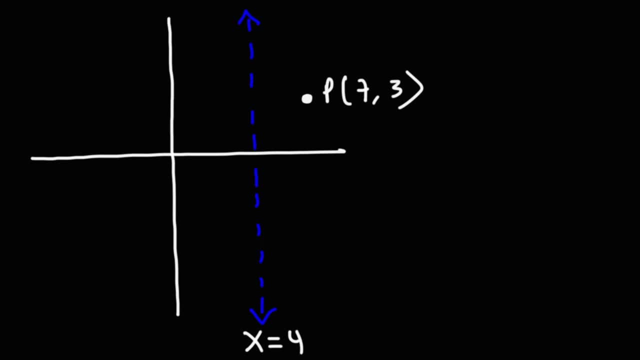 we reflect that point across the line x equals 4?. So that point is 3,, 2, and negative x equals 3.. So we're 3 units away from the line x equals 4.. So to draw the reflected point, 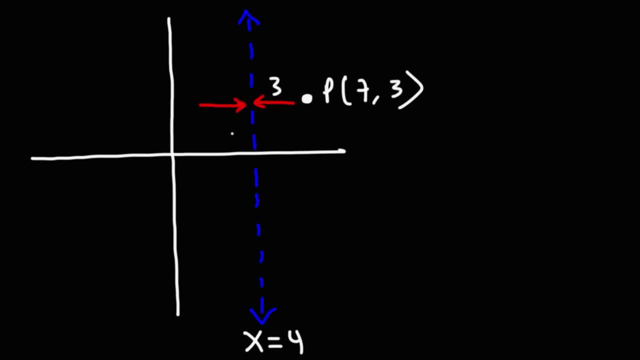 we need to travel 3 units across that line from it. So that will take us to this point. Notice that the y values will be the same for the new point, But the x value will be different. If you want to find the new x value, there's two ways you can do this. You can: 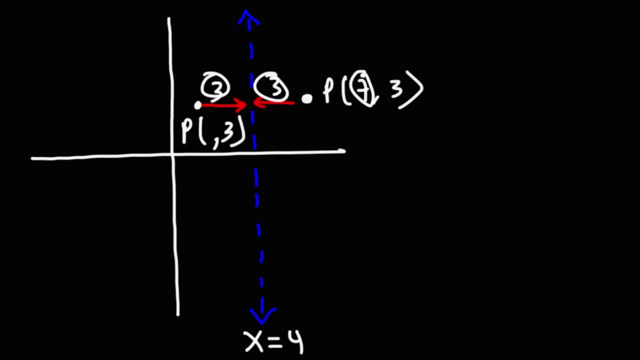 do this by multiplying x by 7 and subtracting it by 3 two times, Which is that's going to give you 1.. That's probably the easier way of doing it. Or you could realize that this 4 is an average of 1 and 7.. So if you set up this equation, 4 is the average of. 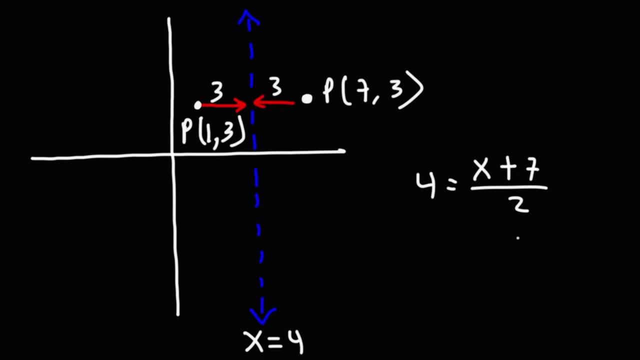 some unknown number plus 7 divided by 2. You could solve for x. So if we cross multiply, we get x plus 7.. So that's how you could reflect a point about a vertical line like x equals 4 or x equals. 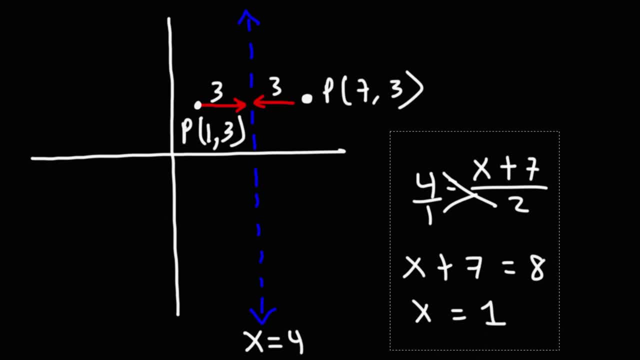 3 or something like that. Now let's do the same thing, but we're going to reflect it about a horizontal line. So let's say we have the horizontal line: y equals negative 5.. Actually, let's make that y equals negative 2.. 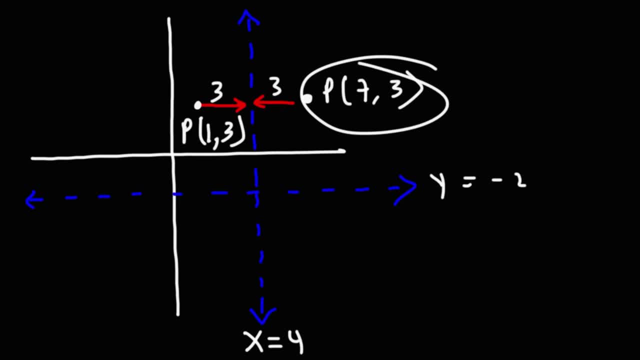 If we reflect this point about the line y equals negative 2, what will be the new point? So let's travel from that point to this line, Going from 3 to negative 2, we're traveling 5 units down. So to get the reflected point, we need to travel another 5 units down, which should: 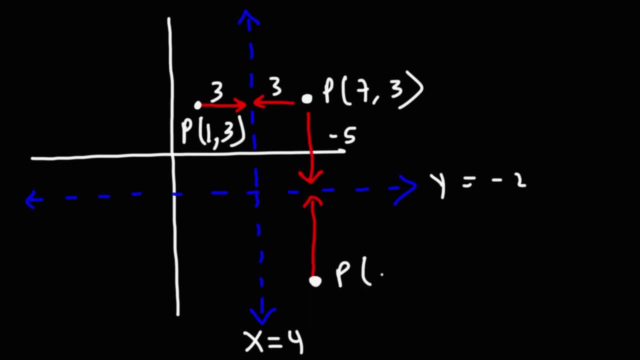 take us somewhere in this region. Notice that the y value is changing. So we're going to reflect this point, which should take us somewhere in this region. Notice that the y value is changing, But the x value remains the same, So it's still going to be x equals 7.. 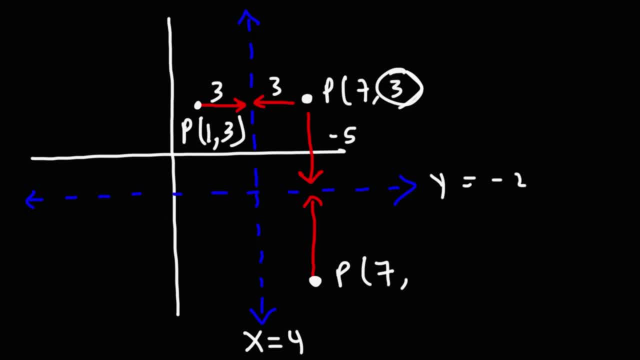 And to get the new point we need to subtract 3 by 5, two times 3 minus 5 is negative 2, and negative 2 minus 5 is negative 7.. So that's going to be the new point. So that's basically it for this video. 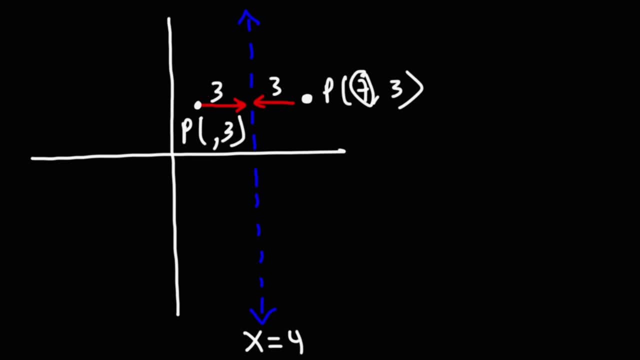 Which is that's going to give you 1.. That's probably the easier way of doing it. Or you can realize that this 4 is an average of 1 and 7.. So if you set up this equation, 4 is the average of some unknown number plus 7 divided by 2.. 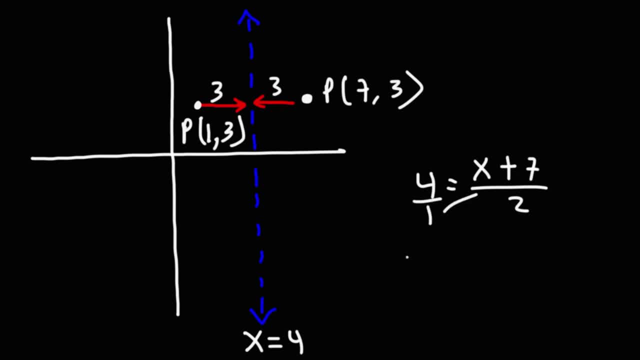 You can solve for x. So if we cross multiply we get: x plus 7 is equal to 4 times 2, which is 8.. Subtract both sides by 7.. 8 minus 7 gives us 1. And we get that point here. 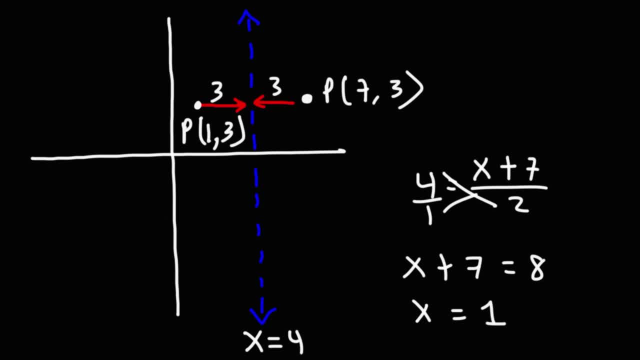 So that's how you can reflect a point about a vertical line Like x equals 4 or x equals 3 or something like that. Now let's do the same thing, but we're going to reflect it about a horizontal line. So let's say we have the horizontal line. 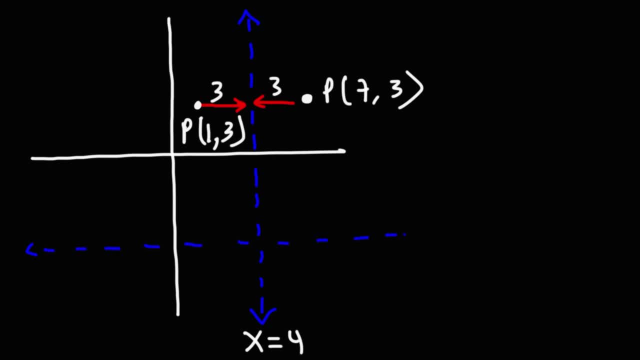 Y equals negative 2.. Y equals negative 5. Actually, let's make that y equals negative 2.. If we reflect this point about the line y equals negative 2, what will be the new point? So let's travel from that point to this line. 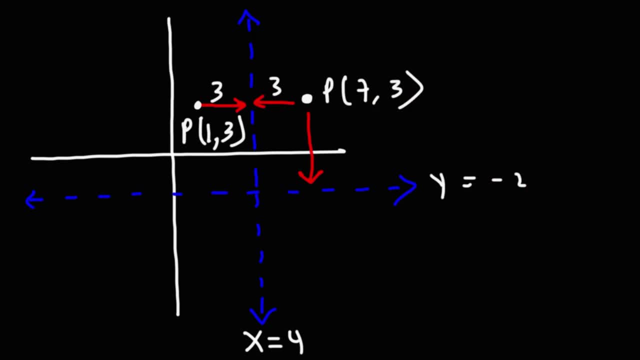 Going from 3 to negative 2, we're traveling 5 units down. So to get the reflected point we need to travel another 5 units down, which should take us somewhere in this region. Notice that the y value is changing. 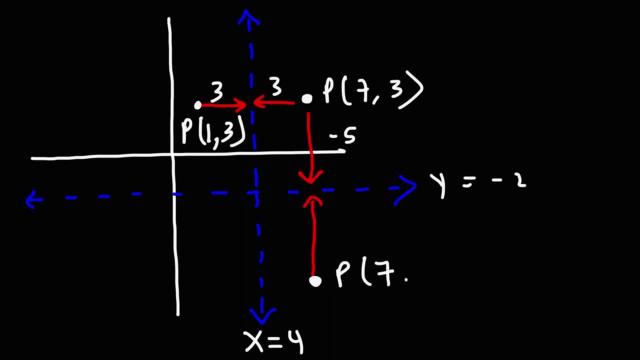 but the x value remains the same, So it's still going to be x equals 7.. And to get the new point we need to subtract 3 by 5. 2 times 3 minus 5 is negative 2.. Negative 2 minus 5 is negative 7..